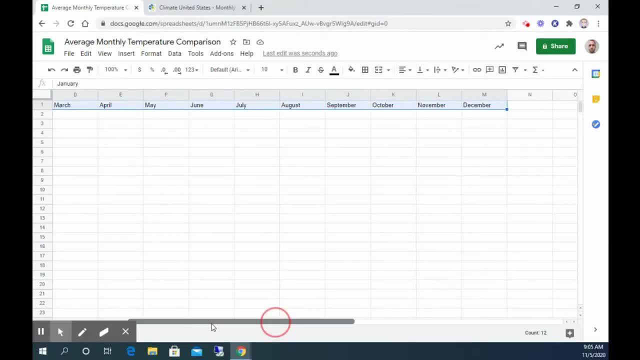 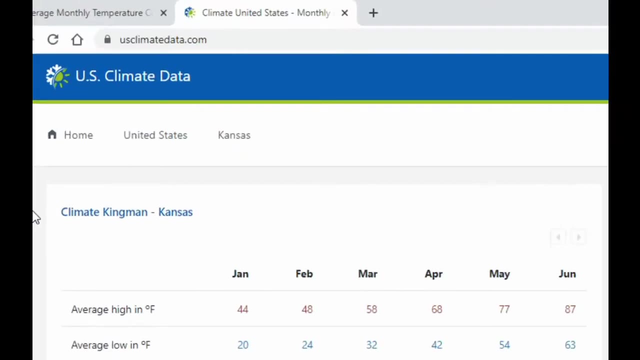 us to December. If you go any further than that, it'll start back with January. So now I have month in A1 and then January through December from B, column B. I also have attached a link to this website. This is where we're going to get our data. 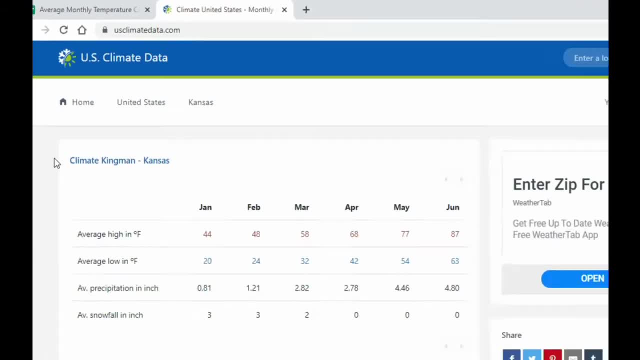 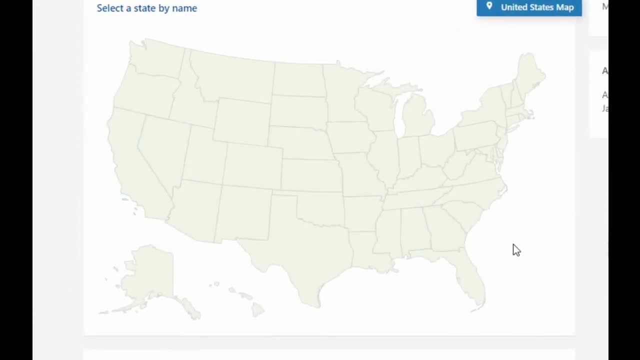 The website is usclimatedatacom And if you scroll down you'll see a map of the United States. It's kind of hard to see because it's a pretty light color, but you can go ahead and click on any state And our goal is to kind of compare two cities that have different. 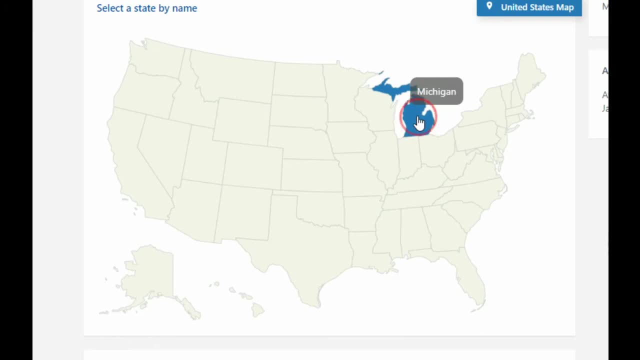 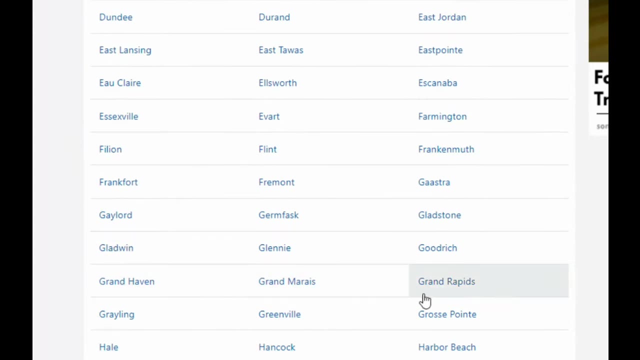 types of climates. So I'm going to go ahead and click on Michigan for my first city or for my first state, And then the city that I'm going to use is Grand Rapids. So if I scroll down, I'll click on Grand Rapids. 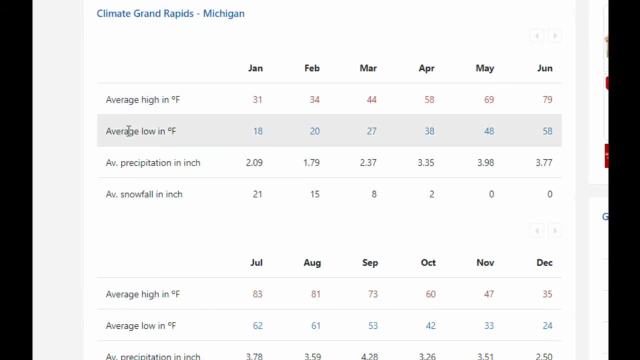 Now it shows me the average high temperature and degrees Fahrenheit and the average low. We're going to use both of these. So we see January, February, March, April, May, all the way to June, And then it continues down here with July through December, So going. 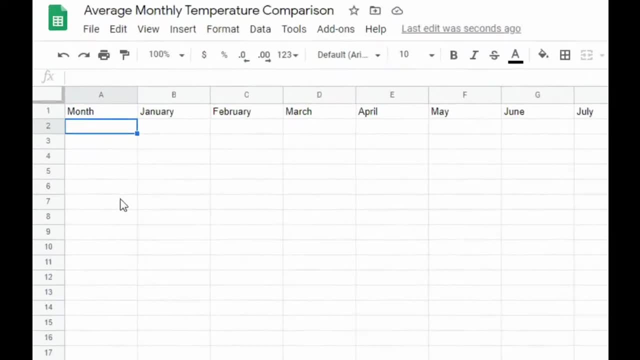 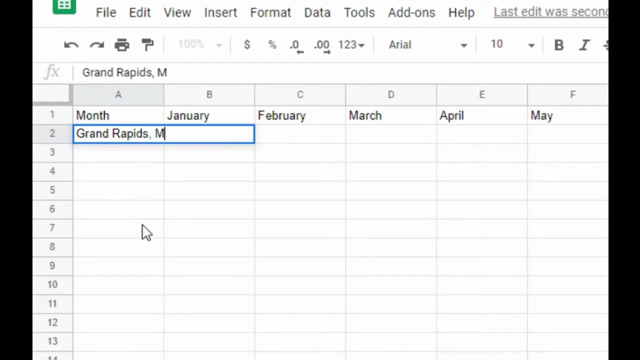 back to my sheet In A2, I'm going to type in Grand Rapids And then I am going to in parentheses I'll put high to remind myself that that's going to be the high temperatures, And then row three, I'll put Grand Rapids, Michigan, and then low. 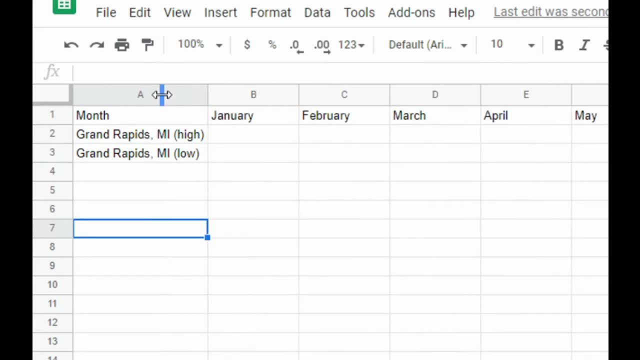 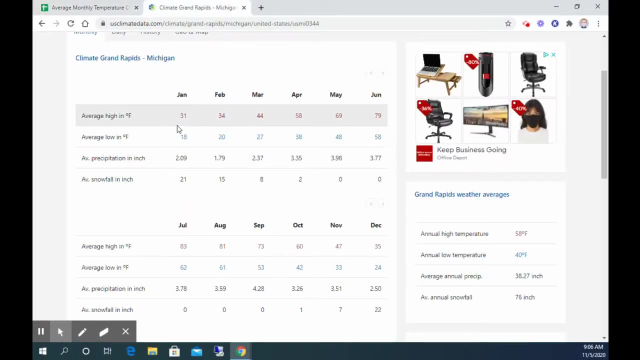 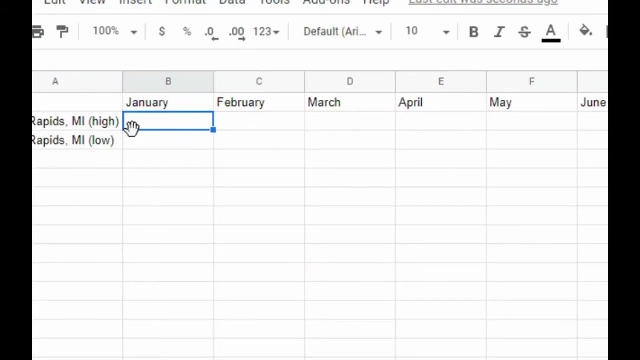 And then again I'm going to want to make my column a little bit wider so all my text fits. So now I'm going to go through and I'm going to looking off this sheet type in the average high for each month. So for January it'd be 31.. February it'd be 34.. So I'll put 31. 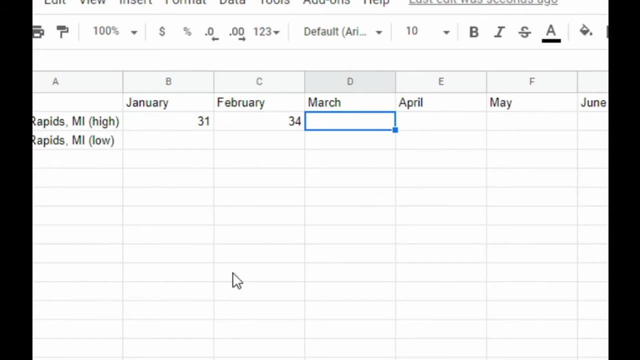 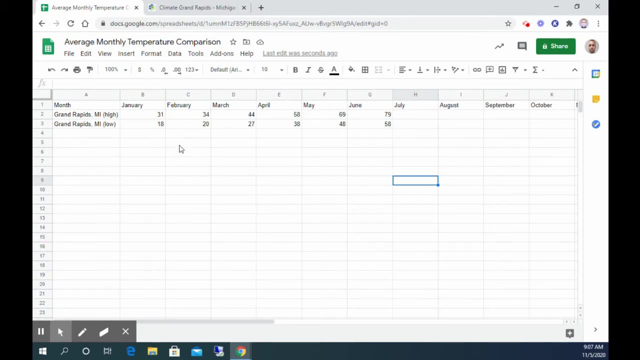 and 34.. I'm going to fill out the rest for Grand Rapids. So I went from January to June just for this example, but in yours you're going to go all the way to December. So now I need to find another city that I want to use, So I'm 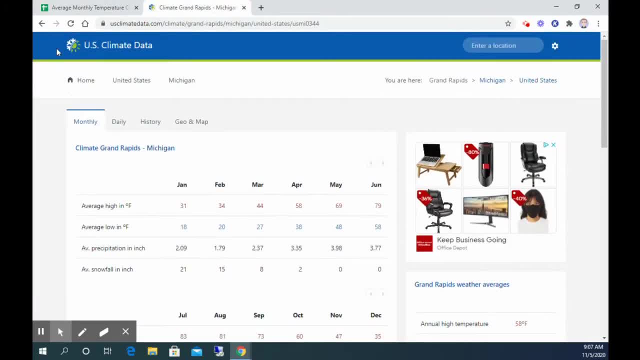 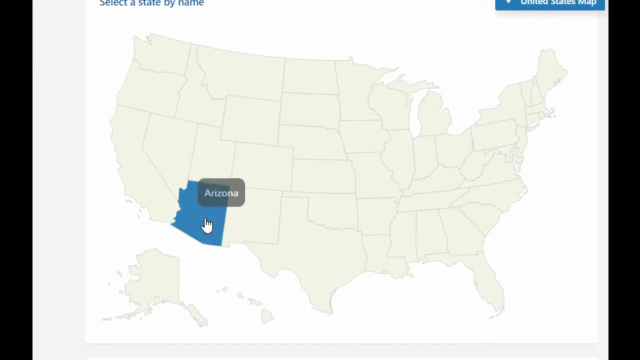 going to go back to my US climate data website, Go back to my map and I'm going to pick another city that I've lived in before, and that city was in Arizona. so I'll click on the State of Arizona And then the name of the city. 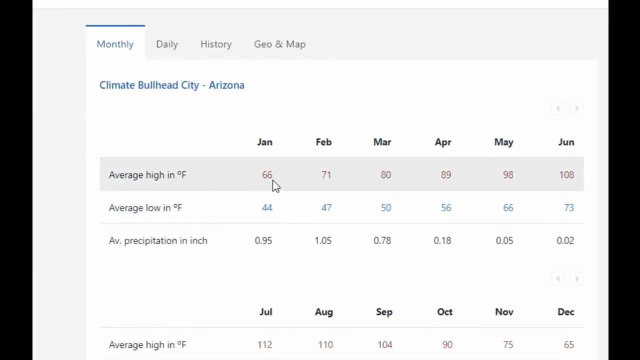 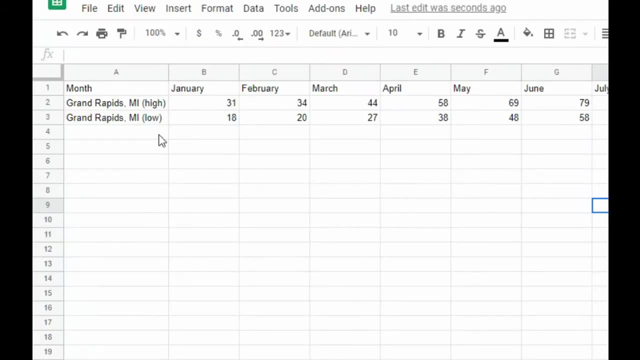 was Bullhead City. And now here I have my average highs and my average lows. So January was a high of 66.. February a high of 71. So let me type in Bullhead City, Arizona, high, and then Bullhead City, Arizona, low. 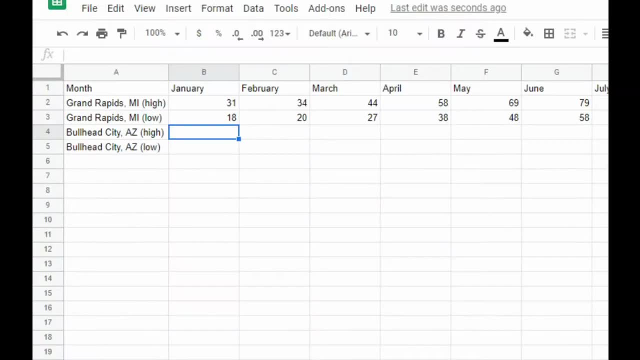 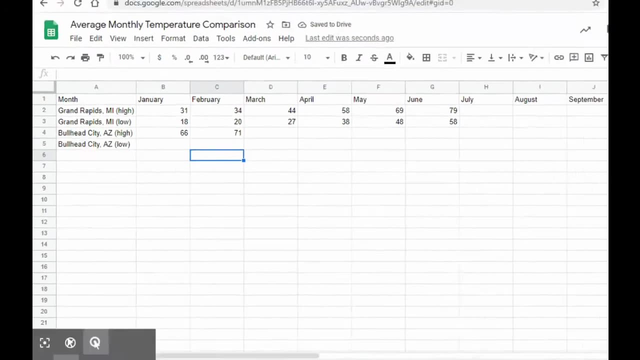 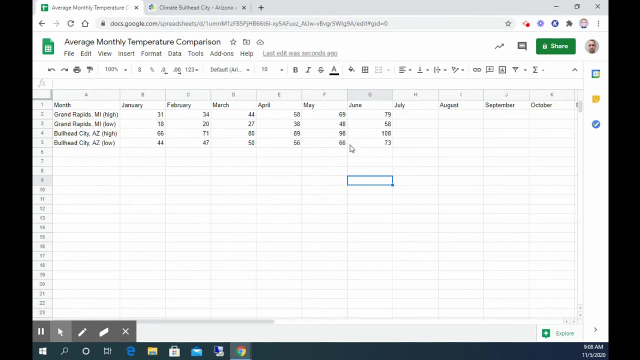 And I said again that was a high of 66 and then a high of 71.. So 66, 71. Now I'm going to go ahead and fill in the rest up until June. Okay, So I have all of my average highs and average lows for two US cities up until June. 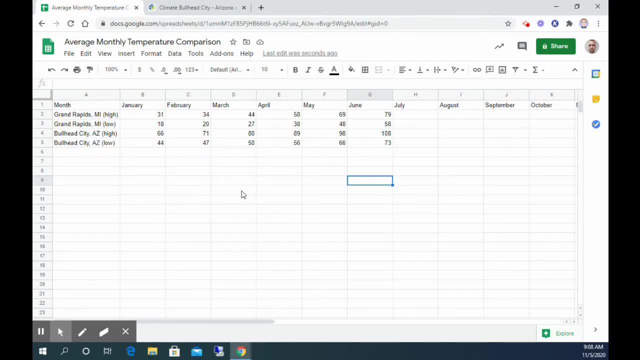 And again, yours is going to go all the way to December, But for this example I'm stopping at June. So now we are going to graph these average temperatures. To graph them, I'm going to click and drag, starting in cell A1.. 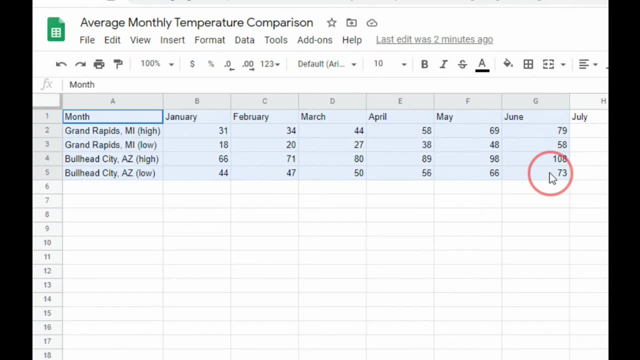 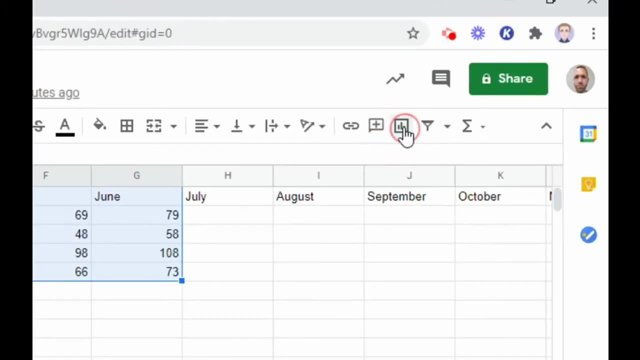 And then I'm going to go to G5. But again, you should be going to M5 to get all of the months After you have them all highlighted in that light blue color, we're going to go to G5.. Insert chart. 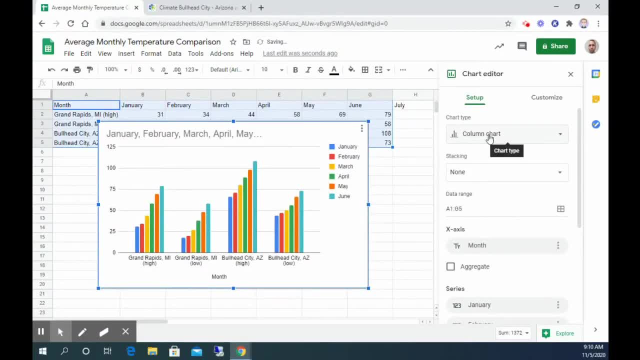 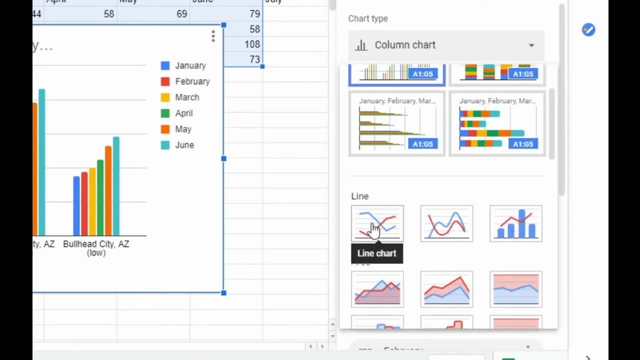 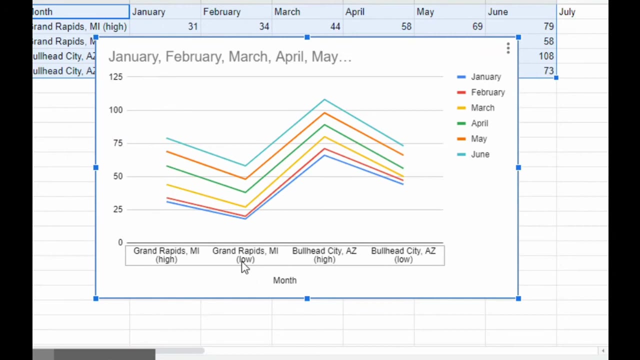 And the chart. we don't want to use a column chart, We want to use the combo chart. So, excuse me, the line chart. So click on line chart And you'll notice it shows our cities on the x-axis here and then our temperatures on the. 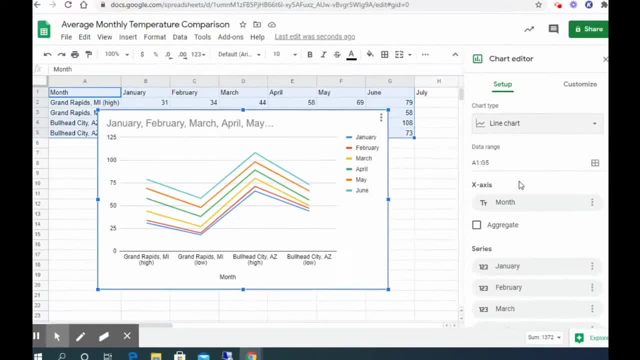 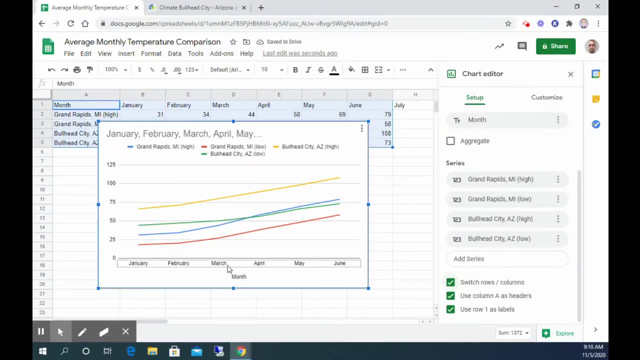 y-axis, So we want the temperatures there, but we don't want the cities here. So if we scroll down, we want to click switch rows and columns And when we do that we can see: Okay, We get our months on the bottom, which we wanted. 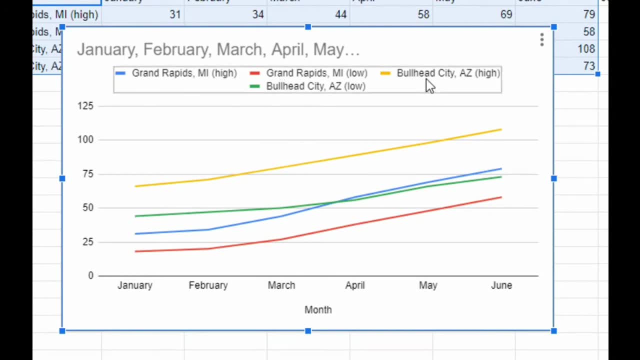 And then our cities are up here showing what color represents each line. So now we can start to edit our chart, So we can double click on the title and we want to call it average monthly temperature comparison, And then you'll notice We've got a y-axis or a label for a y-axis. 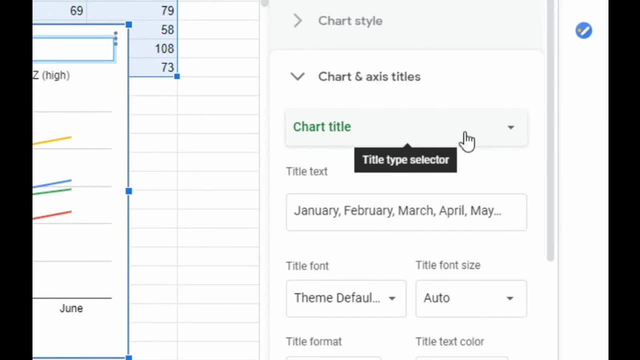 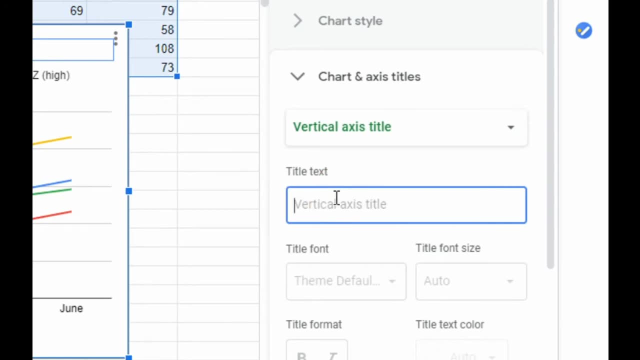 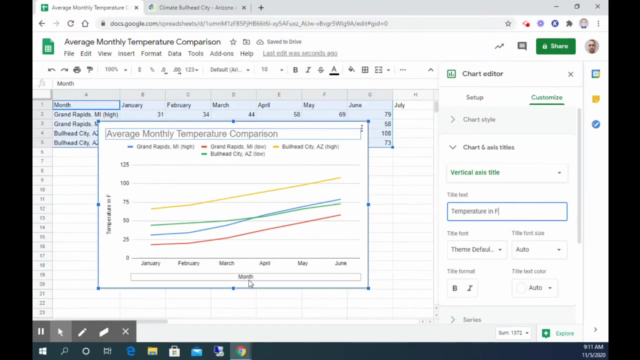 So if we go over to chart and axis titles- right now it's on chart title. If I click on that we can go to vertical axis title, and chart or title text should say temperature and Fahrenheit. So you can put temperature in F and then the x-axis already has the month. 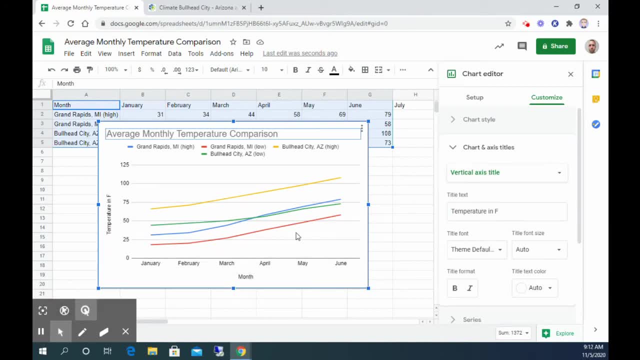 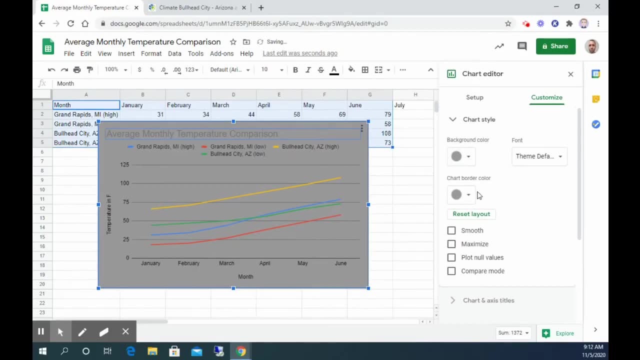 So that one's fine. We're going to change a few more things in our chart, So, if you want, we can go ahead and click on that. Okay, We're going to go ahead and click on chart style and add a background color to your chart. 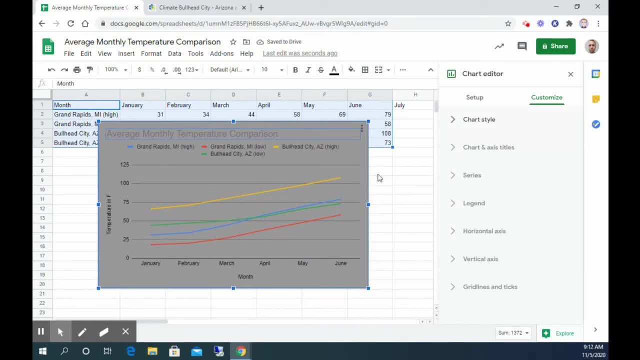 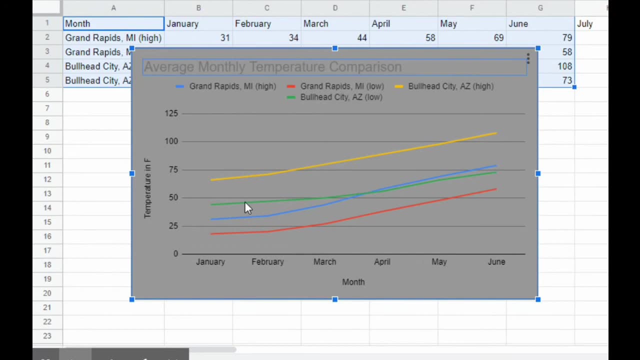 And then a couple of things that we want to do with the lines here. We have a lot of different colors. What I would like you to do is, for each city, I want you to use the same color. So for right now, for Grand Rapids, Michigan, my high temperature is in blue. 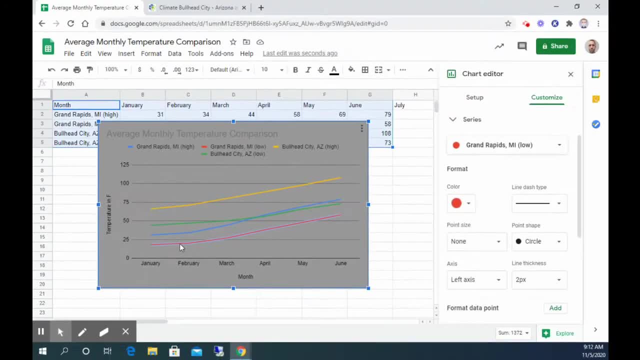 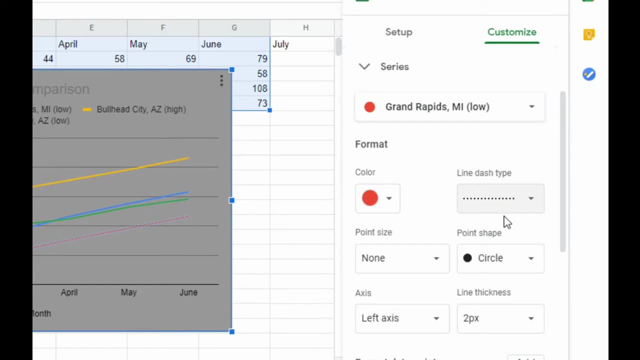 So for Grand Rapids, Michigan, I also want to click on my double click on the low temperature, which is this red line. I'm going to change it. Let's make our lows dotted Okay, Red line, And then I want to change it to the same color that my high temperature was. 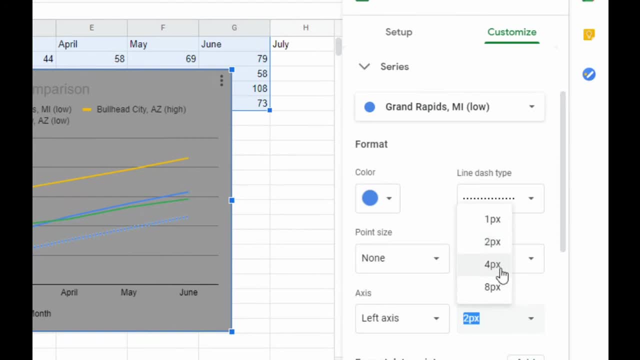 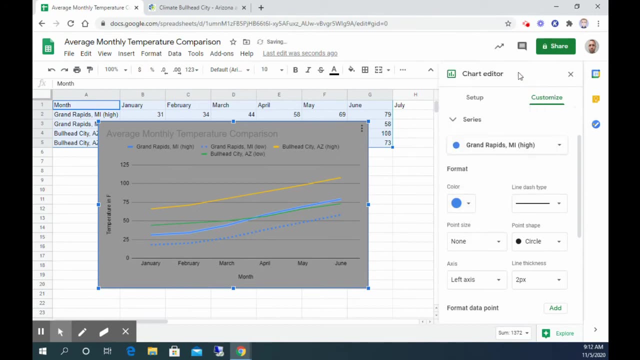 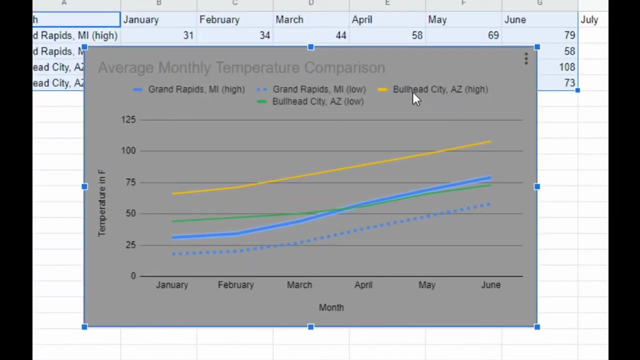 So for Grand Rapids, I have blue now and let's change our line thickness to four, So I have four, and then I'm going to double click and just try to make sure this is the same color and make that four as well. So now for Bullhead City. I'll keep this yellow color, but for my low I want to make it yellow. 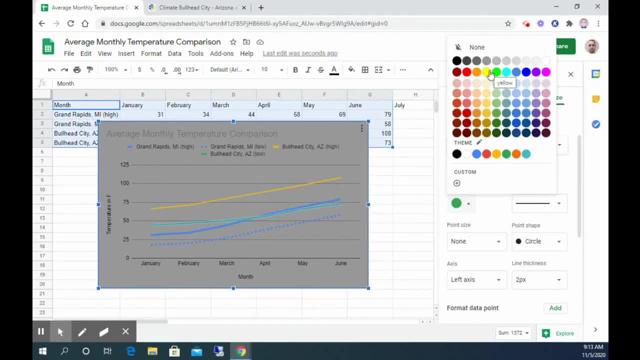 and dotted. So I'll double click on that and pick the different yellow. I'll get those to match in just a second. And then again, the line thickness is four for each one of them. So looking at my chart now, I have- oh, I forgot to make my low for Bullhead City dotted. 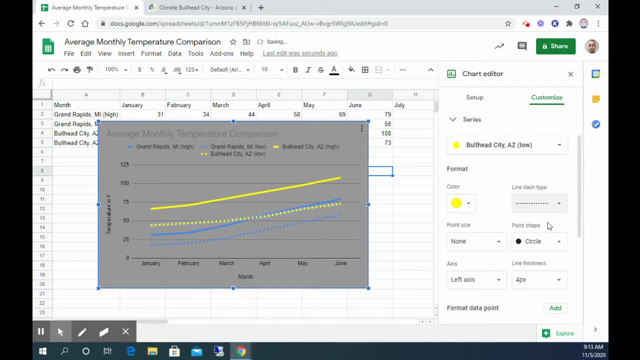 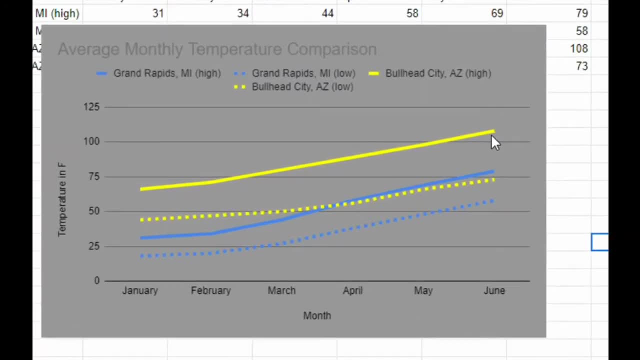 Okay, Okay, Okay. I have a solid line for the high temperature for that city, a dotted line for the low temperature or average temperature, And then again solid for the next city, and then dotted. We're now going to take our chart and we're going to move it to its own sheet. 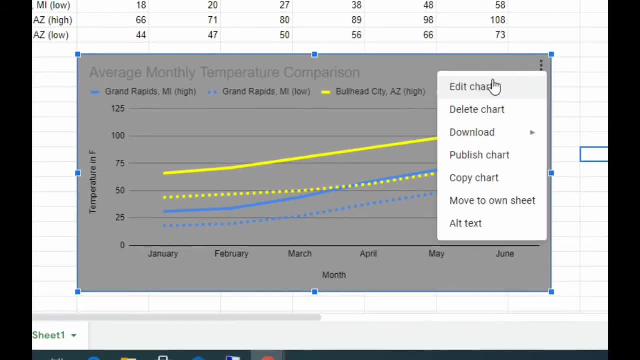 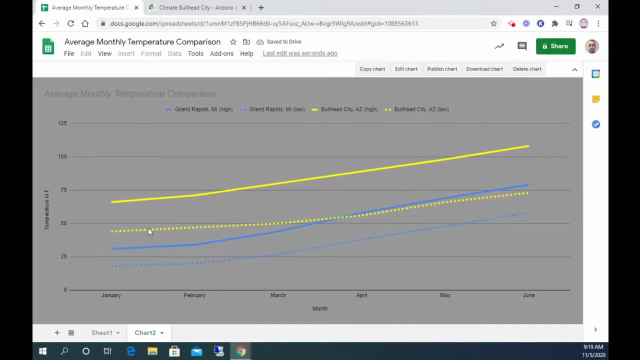 So if you click on the three dots we can go down to move to own sheet And when you click on that it'll create a new spreadsheet that says chart two. Also, like for me, I think. if you notice like your title is kind of tough to read, you can always go down. 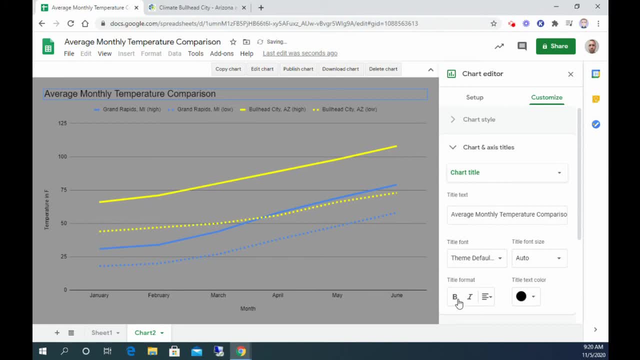 there and you can change the color of that or make it bold so it's easy to read. same with your x-axis and y-axis. if you think those are too tough to read, you can always increase the size of them or make them bold if you need to. so if I 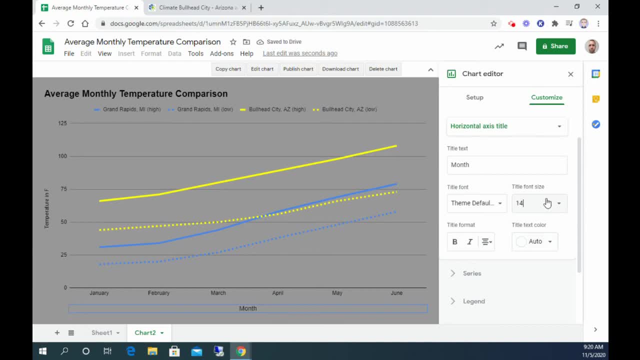 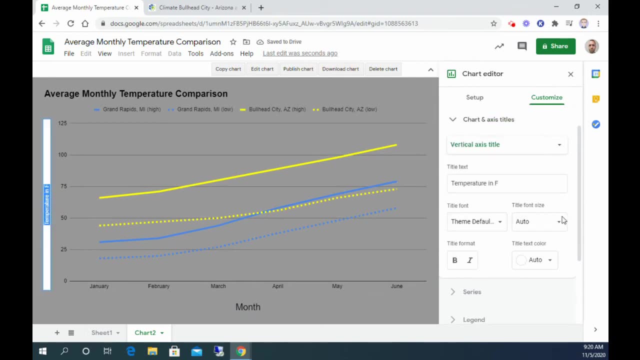 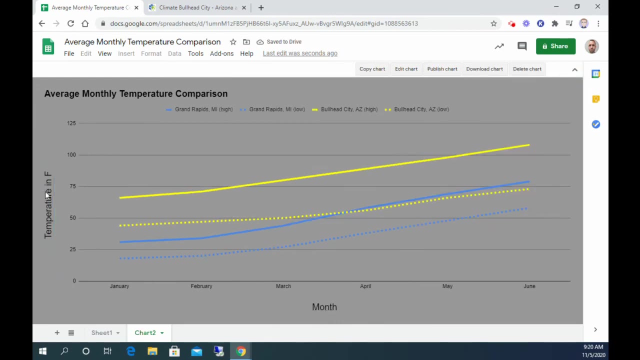 made mine, let's say, 14 size font. it makes it just a little bit easier to read. I'll go 20 and then y-axis, again 20. you don't have to do that, but just as you're creating charts, it might be easier for someone to to view them. so 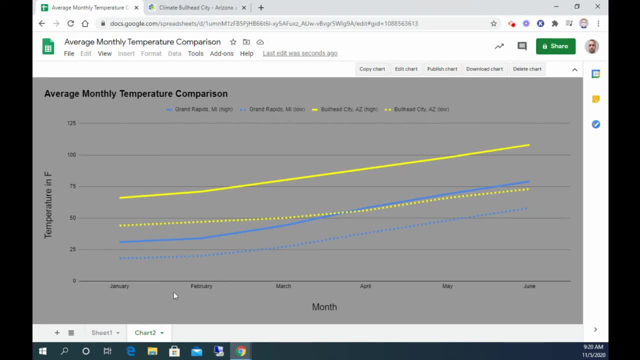 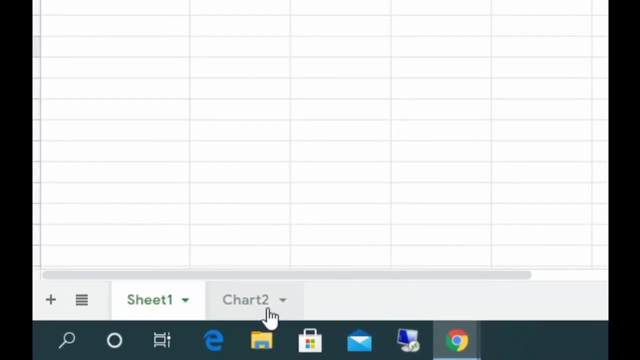 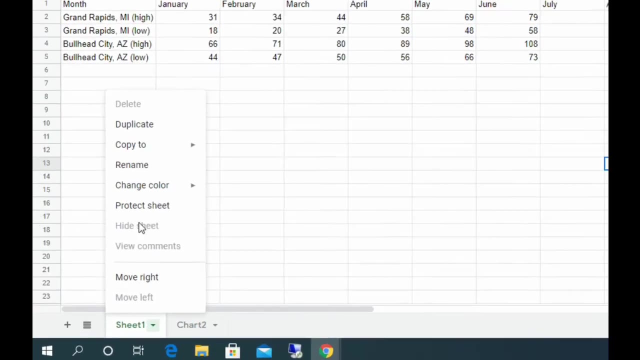 again. yours should go January to December, mine only goes January to June. the last thing we do is we're gonna rename our sheets. so we have sheet 1 which has our spreadsheet information, and then chart 2- our years of price- a chart 1 which has your chart. so let's just right click on it and we're gonna. 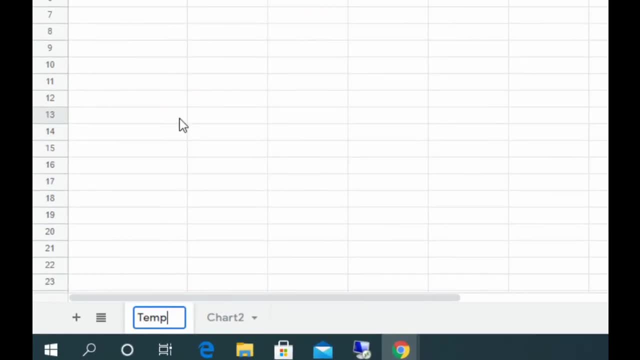 rename it, and then we're gonna go to our spreadsheet and then we're gonna go to our spreadsheet and then we're gonna go to our spreadsheet and then we're gonna name this- we'll call it just temp sheet, and then I'm gonna rename this one and 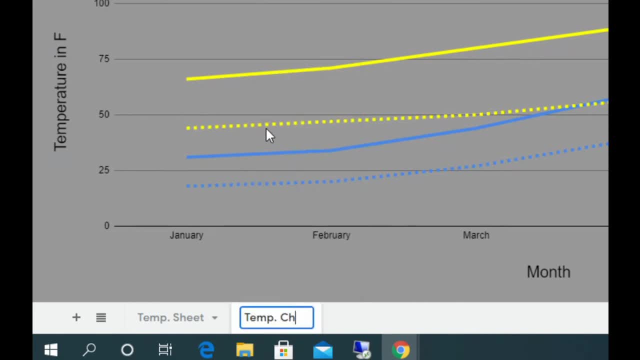 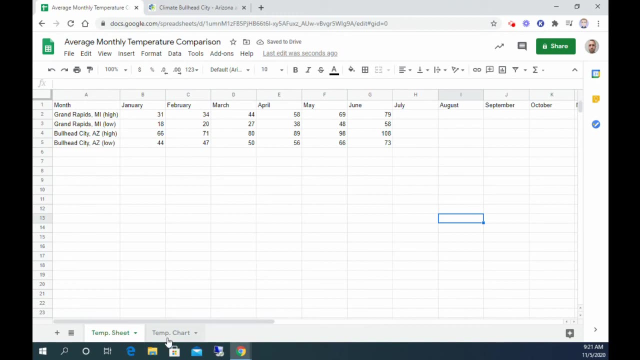 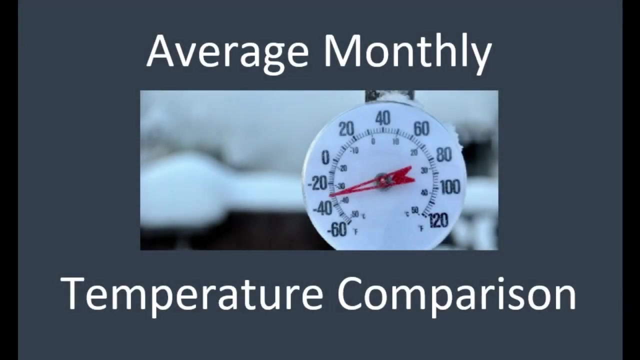 it will say temperature or jump time chart. so now I know, when I click on these, this is gonna be the sheet that, the spreadsheet that has all my data on it, and this is gonna be my chart. so if you have these two sheets and they are complete, you may go ahead and turn it in.